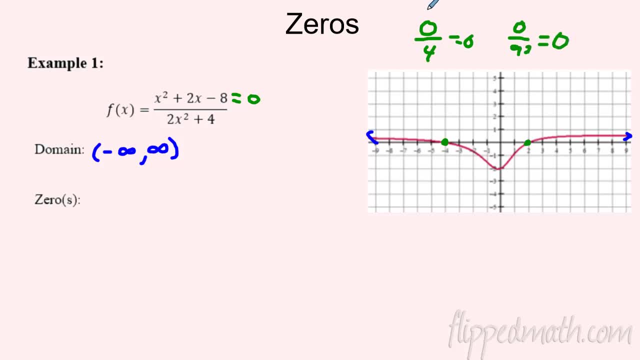 Zero divided by 92? Zero. So again, if the top, if the numerator is zero, the whole thing is zero. Let's get rid of that. Awesome. So let's go ahead and figure out when the top is zero and that'll give us our zeros. So we're going to do a little factoring here. 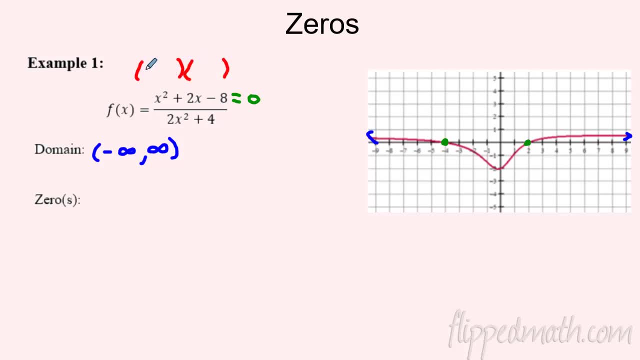 What multiplies the negative eight. As it subtracts to two, it looks like x plus four and x minus two. So we're going to do a lot of little chill factoring here in this section. I'm sorry. this whole chapter, this whole unit. 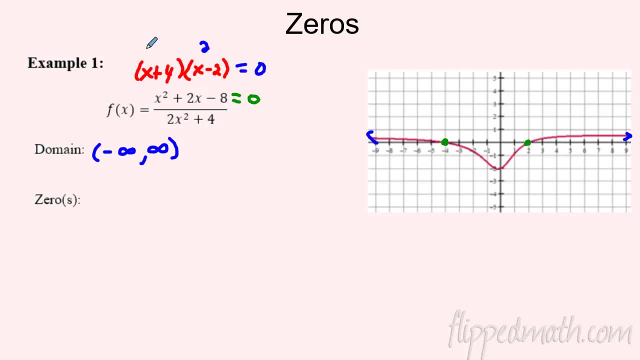 So what would make that zero? Well, that would be if x was two or if x was negative four. Awesome. So where are zeros? Negative four and two. And did that match our graph over there? Sure thing, man. There they are negative four and two. So it all worked out, We're all happy. 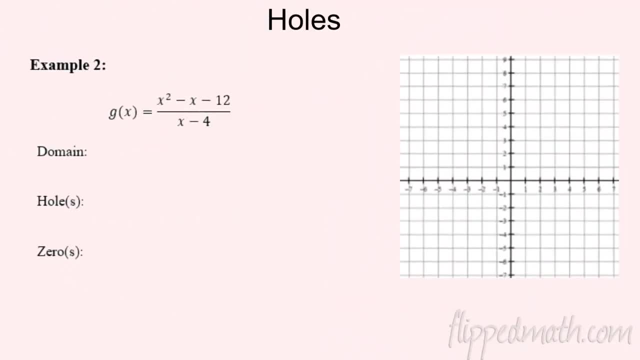 That's the whole section, Holy cow. Well, it's going to get a little trickier. Let's take a look. Some other things can happen. So again, if I quickly look at this, where's the problem with my domain? Remember, the domain is the bottom. I can't have a zero at the bottom. 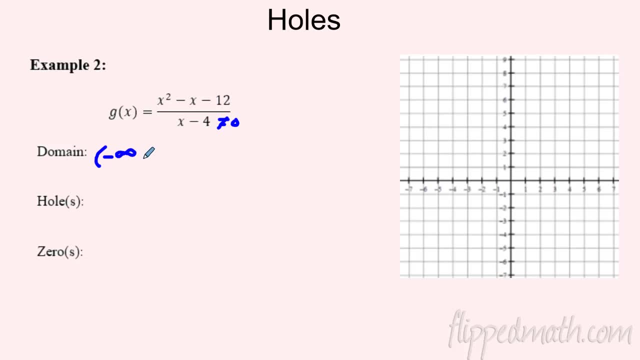 So I can see four is a problem. So everything's cool from negative infinity to four. I cannot be four, And maybe I should add that little union in there and say, okay, it's going to be from four to infinity. So those are the two intervals where the domain exists. 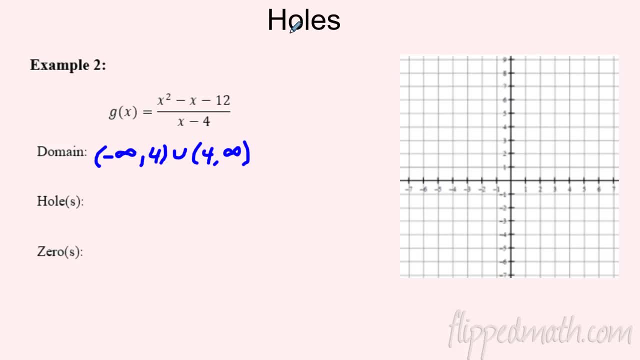 Now I'm going to come back and say, hey, what about the top of this? When does the top equal zero? So on top, I've got what's going to multiply to 12. Let me fix that up a little bit. What's? 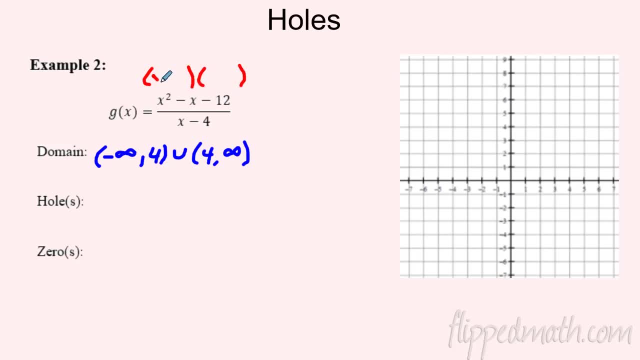 going to multiply to 12? Add or subtract to that negative one here. So if I factor this real quick, you've got x minus four, x plus three. And now check it out. So we've got negative three. Is it possible to place in four? Uh-oh, I've already used four. Remember down here this x. 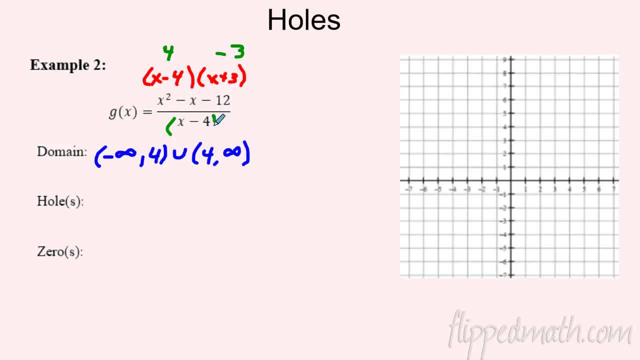 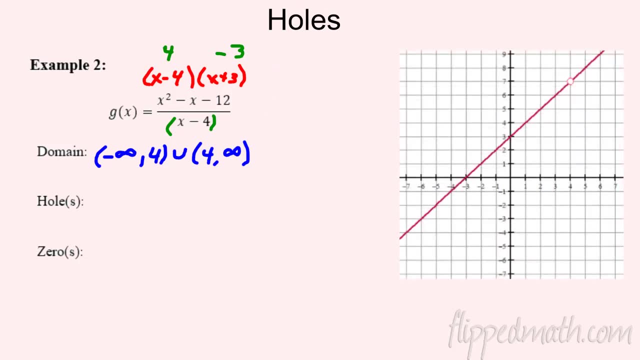 minus four. Oh, interesting, That looked a little rough: X minus four down here. So I've already used it. So what is happening here? Let's go ahead and take a look at the graph. I went ahead to pre-graph this, Oh man. 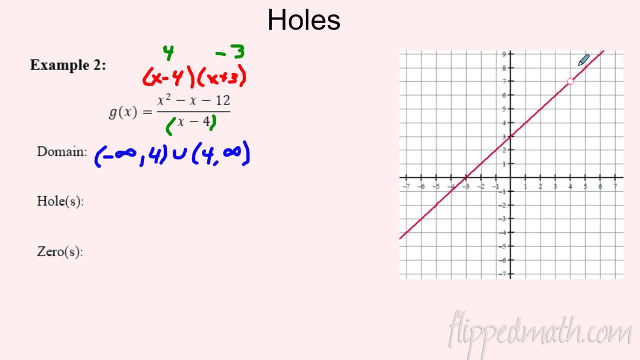 I've actually got a hole, So you have to be careful. We're going to talk where's the hole section, Just a hole section for holes, Chewing that for a while, But there's a. we're going to talk about holes more depth, but there it is. So you can see there's a hole in my graph. Well, 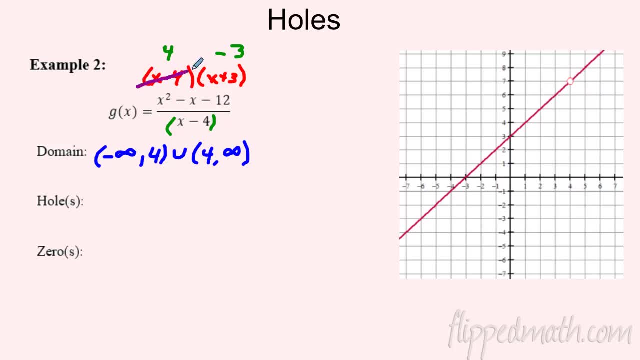 what causes that? Well, if you've got these factors that cancel, so boom and boom, see how these canceled out- That's going to create a hole. So you actually have a hole at x equals four, which means it's not a zero. Even though it's on top, it looks like it'd make the top zero It. 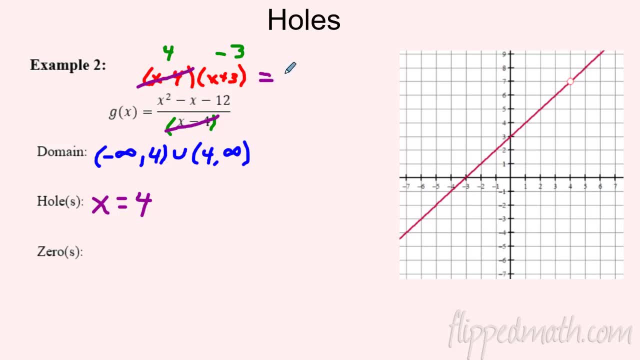 doesn't cancel, So it doesn't work. So the only one who's really making the numerator zero is this negative three. So that's going to be our x intercept, or our root or our solution- whatever you want to call that bad boy or zero, And you can see him right here. So you just have to be careful. 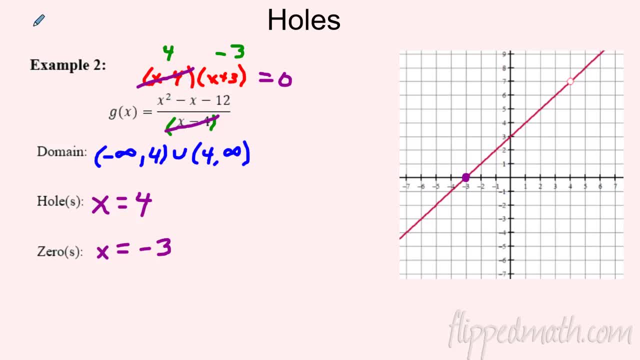 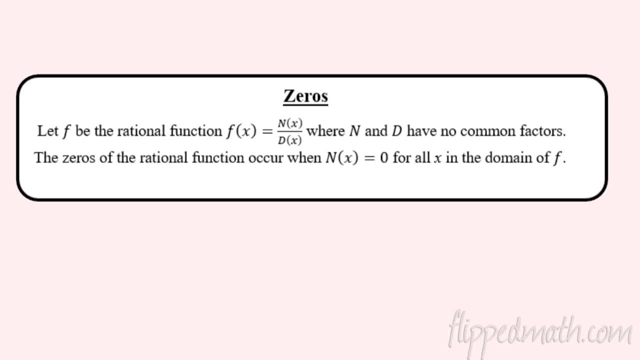 that it doesn't cancel out. Long story short, if it cancels out no longer a zero, That's two examples. It could be record time. I love formal definitions, So here's the formal definition of zeros. Basically, what did we just talk about? They cannot have any common factors. The zero. 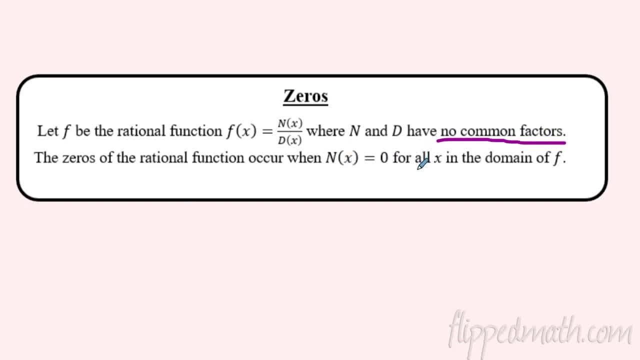 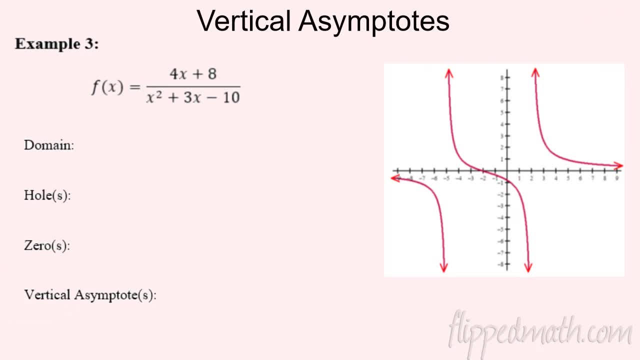 happens when the numerator is zero, when the top is zero, but they can't have any common factors. that cancels it out. All right, here we go. Let's look at the next example. Ooh, now we got to worry about vertical asymptotes here, So don't freak out, There's going to be a whole section on. 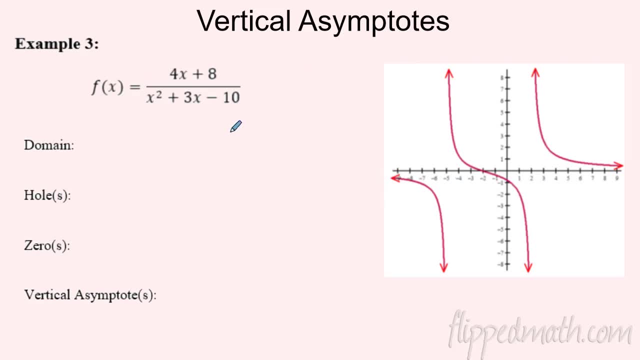 vertical asymptotes And I went ahead and I graphed it for you so we can kind of see what's happening here. But there's other things that may cancel. So we don't always have holes. Sometimes they do, But really everything starts off the same. We're looking for: okay domain, No zeros. 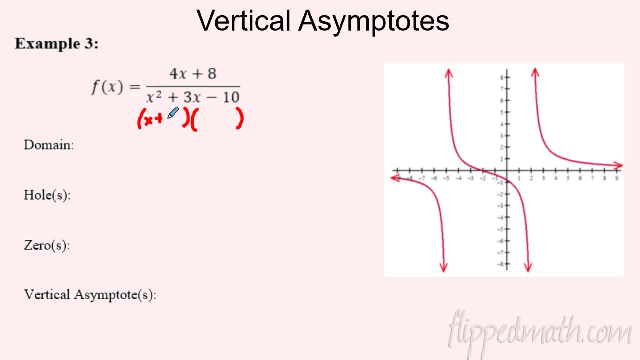 in the bottom. So quickly, let's factor this: What multiplies to give you 10 and adds or subtracts to give you three. Looks like I think it's five and two. Is that cool? And then does the top factor anything in common? Sure, They have a four in common. So I'm going to say four and pull that. 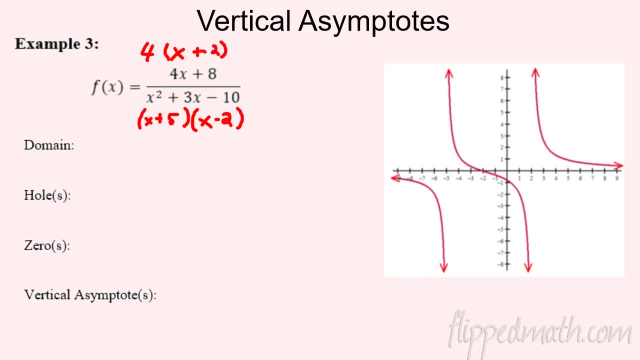 out, You get X plus two- Awesome. So if I'm looking at where my issue is, negative five is going to be an issue and two is going to be an issue and negative two. Oh, did they cancel? Does anything cancel? No, So I'm going to say four and pull that out. You get X plus two Awesome. So if I'm looking at where my issue is negative: five is going to be an issue and two is going to be an issue and two is going to be an issue. I'm going to say four and pull that out. You get X plus two. Awesome. 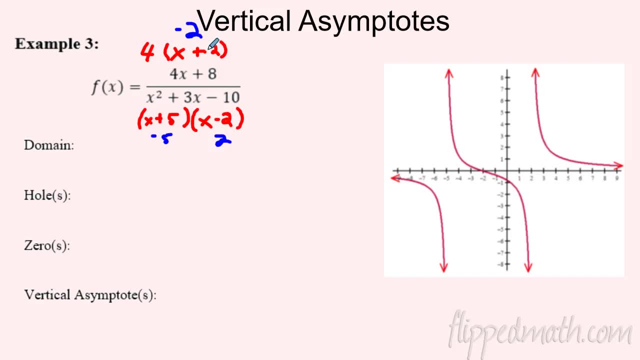 It's close, but we've got a negative two and a positive two. These factors aren't the same: X plus two, X minus two, Not the same. So we're cool there. So for domain, what's happening with the domain? I'm going to be everything from negative infinity to negative five in union with the next. 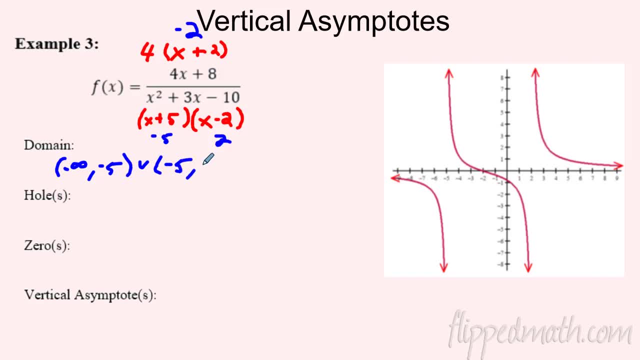 interval I can see it's from negative five to two. I'm cool if I go there And then in union with the last interval, from two to infinity, And I went ahead and pre-graphed this for us so we could take a look at it. Does that make sense? No, So I'm going to say four and pull that out. 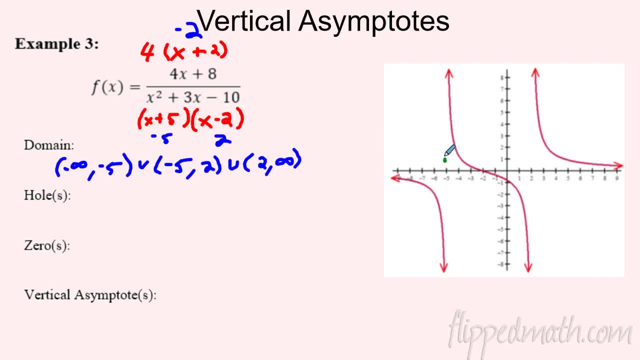 Does that make sense? Sure, Everything is cool until I hit this negative five, and then I get this vertical asymptote. Draw that little bad boy in there if you want, We can see there's a problem, and then at two there's another issue. We've got another vertical. 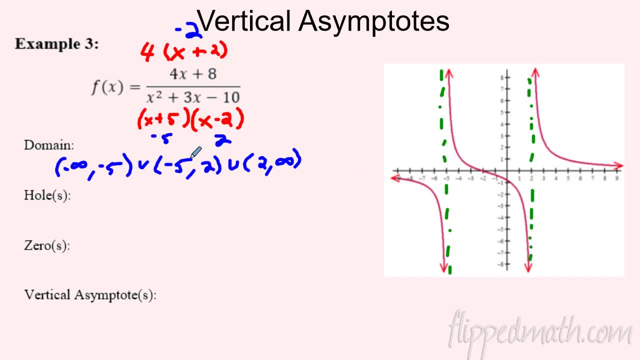 asymptote right there. So we're kind of looking for problems and we found them There. they are All right. Did any holes happen? Did anything cancel? No, So we don't always have holes. That would just be if something cancels on top and bottom. I've got no holes in this one. We're. 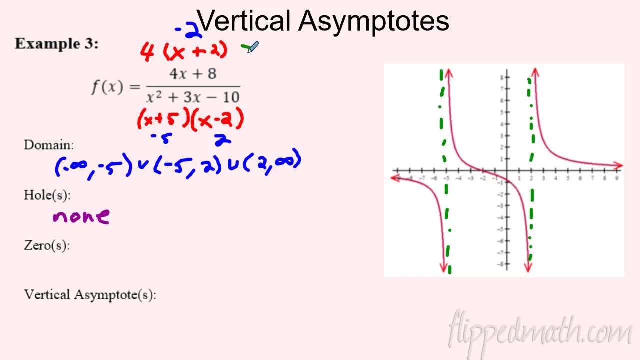 pretty cool on that. How about zeros? Again, the zeros is when the top equals zero. So does that ever equal zero? Sure, Negative two. We already solved that. factored and solved it. We get negative two on top. Does that match my graph? Yeah, there, it is right. there, I can see that. 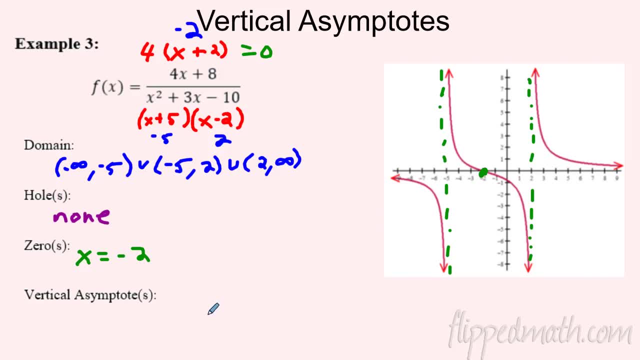 bad boy with a big old dot right there And do we have vertical asymptotes? Yes, we have vertical asymptotes. So it's these places on the bottom that didn't cancel. It's when the bottom equals zero. When that happens for domain, we say it can't equal zero. When it actually does happen. 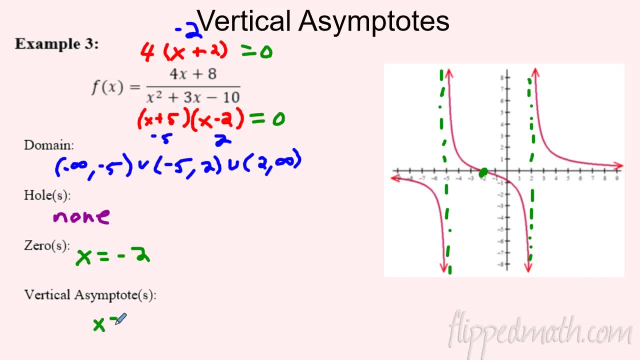 that's cool. So we're going to have a vertical asymptote at negative five and two. So again, basically, we're going to factor everybody: If it doesn't cancel, it's going to be a vertical asymptote. If it does cancel, it looks like it'll be a hole for now. Awesome, We are cruising That could be. 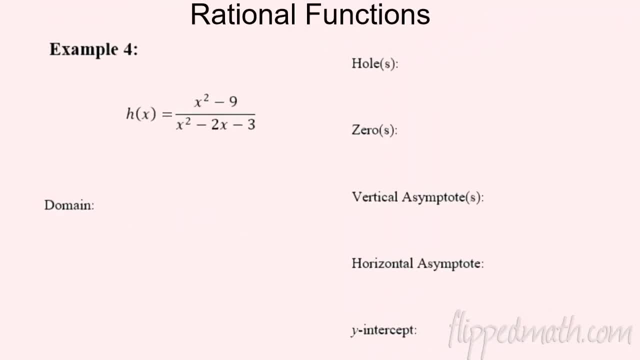 a record here, So let's do without a picture. I have no picture to go on. If you want to pause it and try it and see how you do, that's cool. I'm going to go through it quickly with you so we can just check it out together. 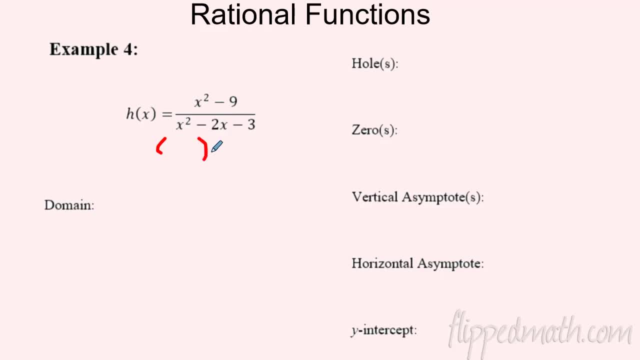 Let's- I'll go in order here. Domain. We're looking at the bottom, So let's do a little factor factor. I like that. What multiplies to three. Only one thing that multiplies to three. We're going to do negative three and one. Sometimes they're so easy, they're hard. 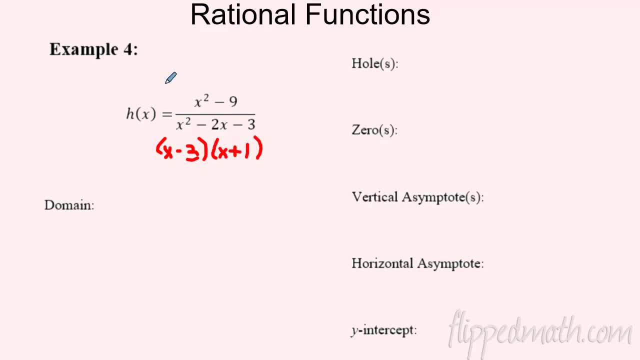 Only one thing it can be, but it looks weird On top. that's a difference of squares. So we've got x plus three, x minus three. So I always start off just say, hey man, let's factor it and look. 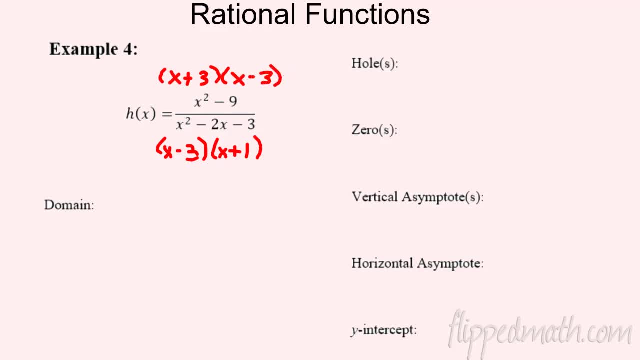 for any cancellations. So is anybody going to cancel here? Yes, we have an Issue at negative three. So does that matter? for domain Domain doesn't care. There's issues everywhere from domain. The domain is just that bottom. The bottom can't equal zero. So when I do, 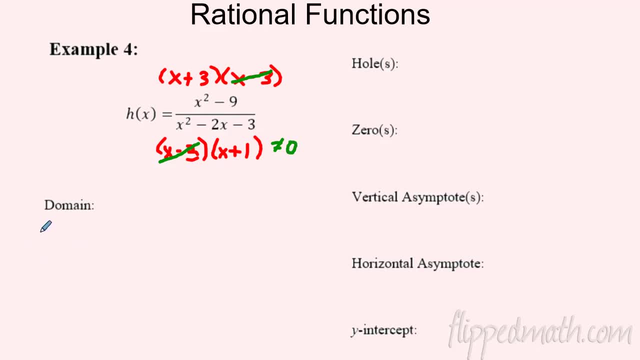 this on bottom. he's going to say, yes, we have issues at where negative infinity to me. I should put some numbers here. We have this problem at three negative one. Remember that three on top was the same in negative three. That's where all our issues are. Again, domain doesn't care in the 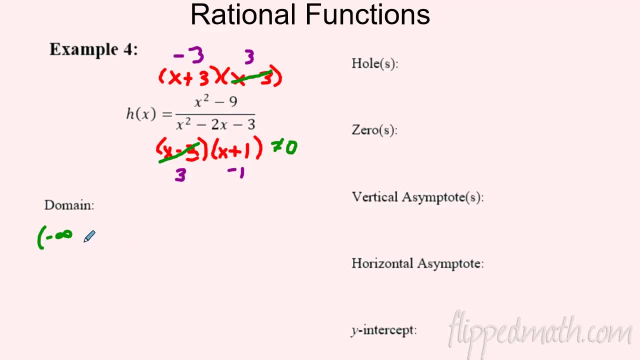 bottom. If you're a whole or A vertical asymptote, he doesn't really care, He just knows there's a problem there. So we will be cool from negative, negative one, And then we're going to go from negative one to three. So it's. 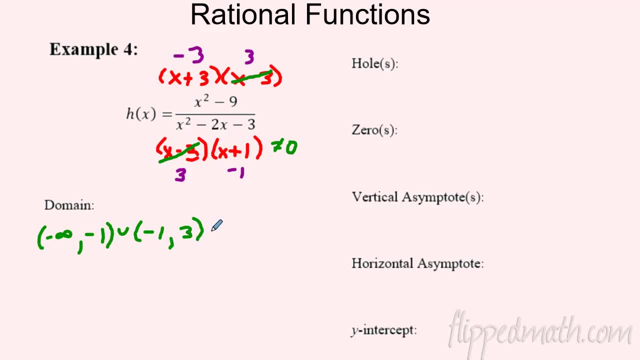 just the bottom. I got too excited, I canceled that out too early. I just get too fired up to do these. And then we're going to go three to infinity. So cancel, no, cancel. Who cares for domain? We've got problems down here. So we identify the problems of domain. There's going. 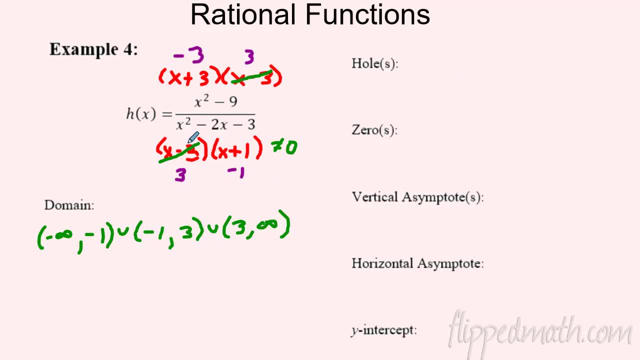 to be breaks in the graph. Is there a hole? Yes, I already canceled it. I got really excited there. There's a hole at three Because it canceled, So that's going to cause some kind of hole in the graph. Just draw a little. 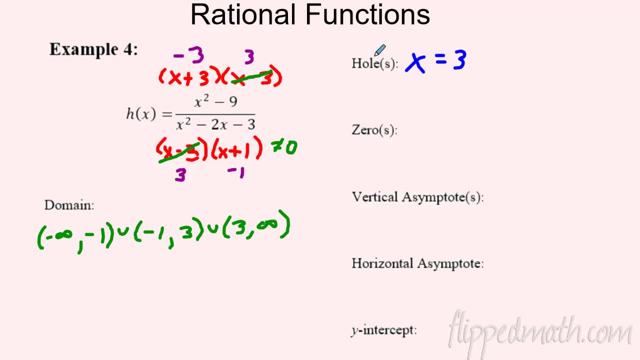 open circle If you had to graph it there. The zeros: Are we going to have problems with zeros? The zeros at the top. So this is a hole. Holes can't be zero, So we can't even mess with him. 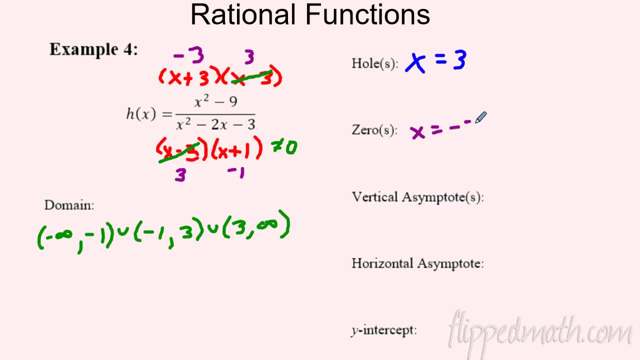 But that top is negative three, We'll make the other one. We'll make a x-intercept because it makes the top zero. So we're looking over here. When the top is zero, it's this one. Excellent Vertical asymptotes, Do we got some? Well, that's a hole. We already labeled that a hole, So it's. 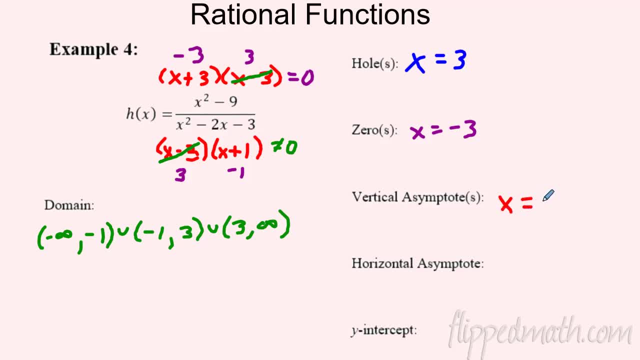 the other guy over here. We're going to say x equals negative one, And again, we'll get way more in depth on these later in the next couple sections. But we got to be able. they're going to be a problem because they. 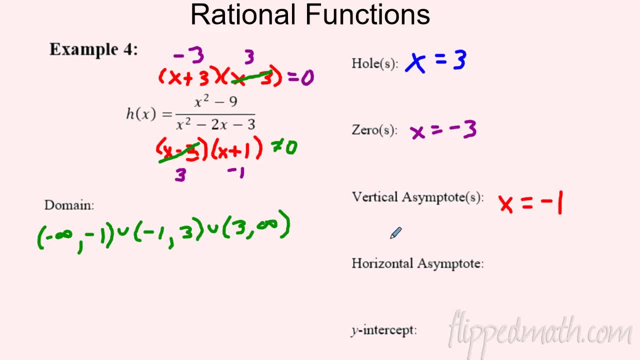 mess with our zeros. Excellent. So we've got that vertical asymptote with negative, one Horizontal asymptote. Oh, this is old school. Going back to last section, So we're now looking at the limit to infinity. So I look for the high power. So you see the high powers right here. 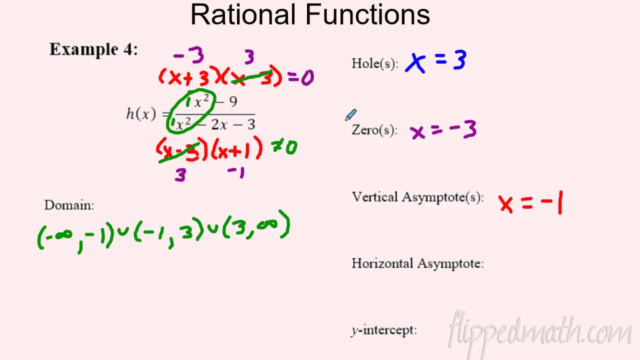 They are going to be the same. So it's one and one The highest power. So I know that gives me a horizontal asymptote. at one. We're looking for bigger in the top, bigger in the bottom, or the same. And then y-intercept What happens if you plug zero into this equation. I mean you can go. 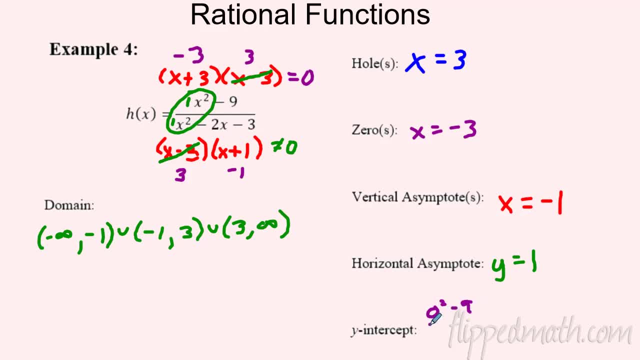 ahead and do that. You can say zero squared minus nine, all over zero squared minus two times zero minus three. But when you're plugging zero in to find that y-intercept what's going to really happen? You're going to get a lot of canceling. Zero is just zero, zero two times zero zero. 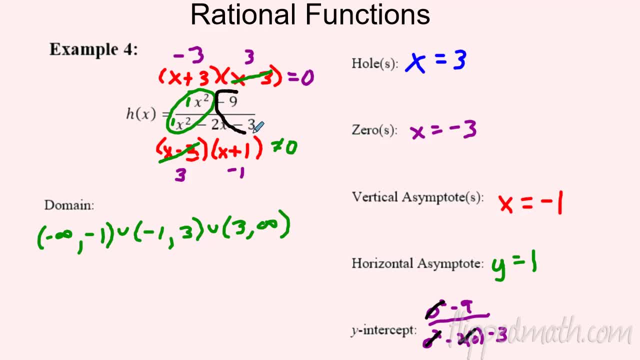 What are you left with? You're just left with this last part. the constant, the negative 9 over negative 3, and negative 9 over negative 3 is just 3.. That's the y-intercept. If you'd like to write it as a point, you can put it as 0,, 3, but a lot of times we say the y-intercept is 3.. 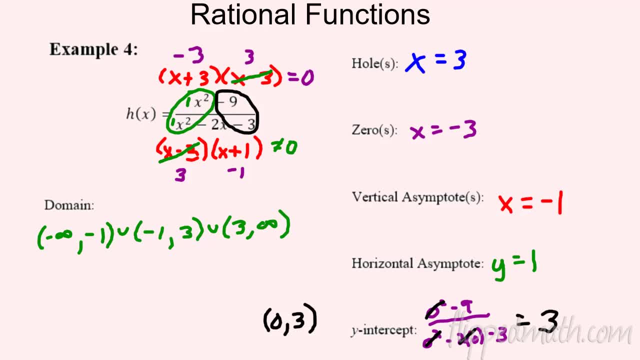 That's where this bad boy starts. Awesome, That was it, man. If you can do that, you're going to crush this. So it's a lot going on. Our main focus is 0, but the hole's kind of messed it up, because you could actually get a hole right there on the 0 and it doesn't count. 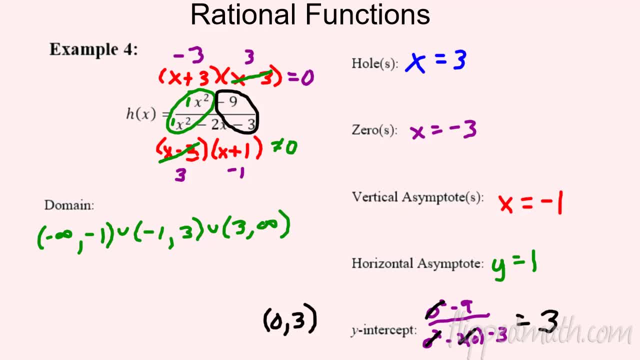 And then vertical asymptotes happen. so might as well, let's just talk about them now. Rock and roll, Last one with a graph, though, just to make sure, graphically maybe I don't give you an equation, so you can't do all those fun rules. 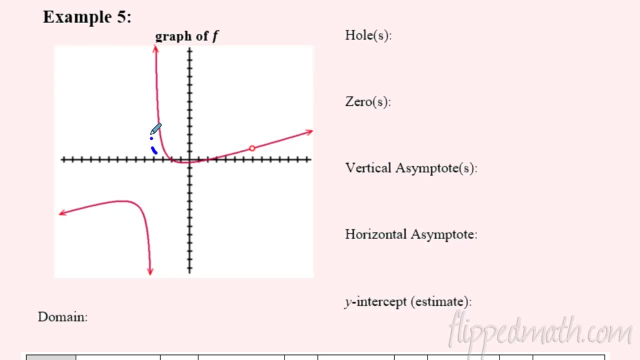 Can you just look at this? And for these pictures we're going to go ahead and say these are vertical asymptotes. Sometimes I draw them in, Sometimes I just say, hey, it's going to be 1.. There, it is right there. 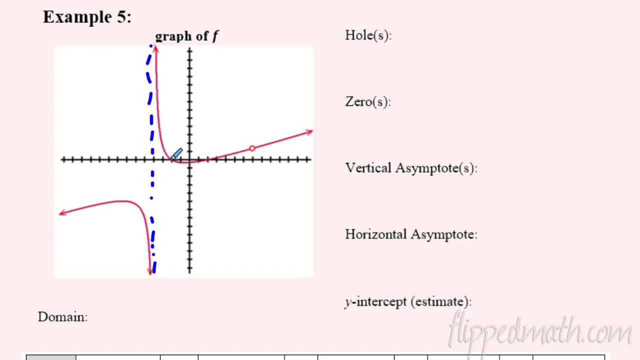 So we've got issues there. I can see that little hole right there. I can see some other things happening here. It looks like it's crossing right here and right here. So can you label all these points? Sure man, Let's do it. 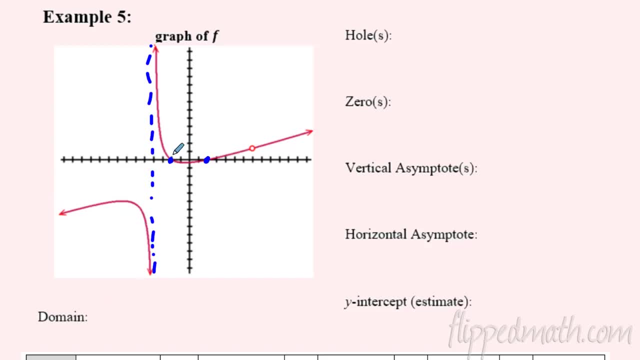 So the domain is very smooth until I hit what is that? 1,, 2,, 3,, 4.. Looks like 4 is my first issue. So it's kind of like: where do I have to lift my pencil first? I'm going to have to lift it at negative 4.. 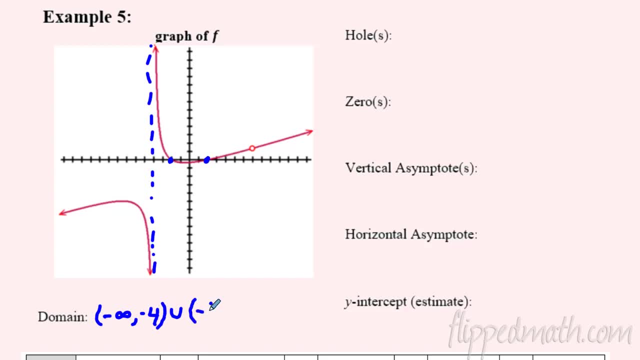 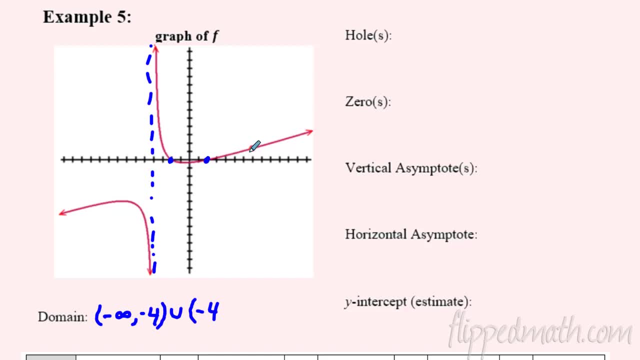 I had to lift my pencil. Don't worry about zeros, Who cares, You're just chilling, chilling, chilling, Uh-oh problem hole. So I had to lift my pencil here and then I can put my pencil back down. 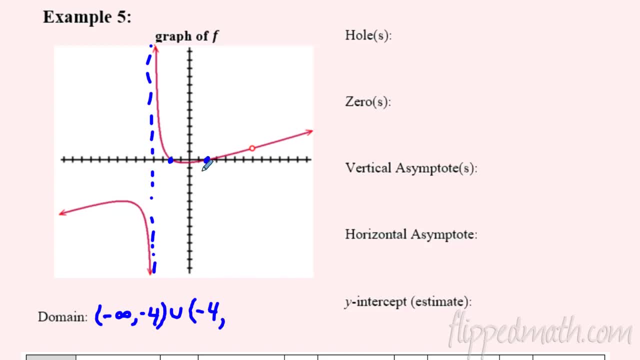 So anywhere you lift that pencil is a problem for domain. Where does that happen? out here It's 1,, 2, 3, 4, 5, 6.. That looks like 7, I think out here. Hope I can count right. 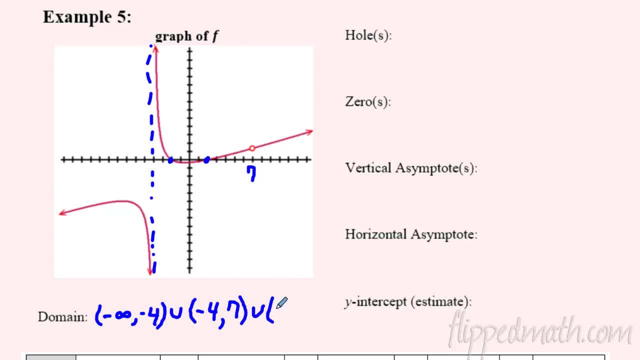 And then the last interval where it just kind of flows is 7 to infinity. Awesome, So it's continuous on those intervals right there. Excellent, Where was that hole? I can see it right there. We just counted that out: x equals 7.. 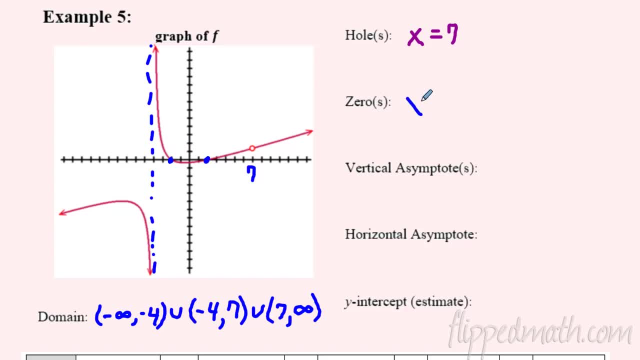 Where are those zeros? Where does it cross? It looks like negative 2.. I love it when it's a picture. It looks like x equals negative. 2 is the first zero and the second one is where Negative 2 and positive 2.. Excellent. 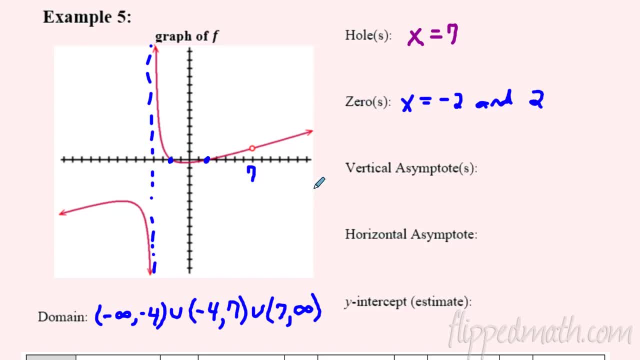 So those are where it crosses the x-intercepts. Is there a vertical asymptote? Sure, I drew that in there. We've got that happening at negative 4.. 1,, 2,, 3,, 4.. And then, is there a horizontal asymptote? in this case, No, I don't see a flat line. 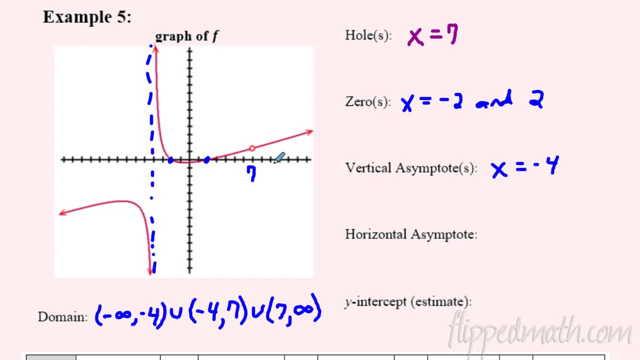 It kind of goes forever and ever up, forever and ever down, as I look at the end behavior. So there is none. That's totally cool. You don't have to have everything. You can't get everything you want. And then we're going to estimate the y-intercept. So where is that y-intercept? It's right here. 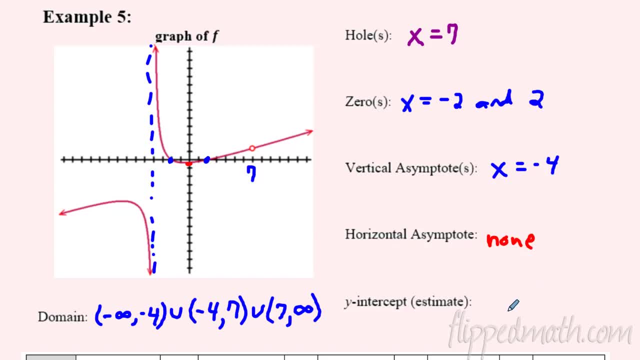 It looks like it's not even a half. So it looks like I don't know. I'm going to say approximately negative 0.3.. So roughly it looks like it's that negative third right there somewhere around that. Awesome. So graphs are great.